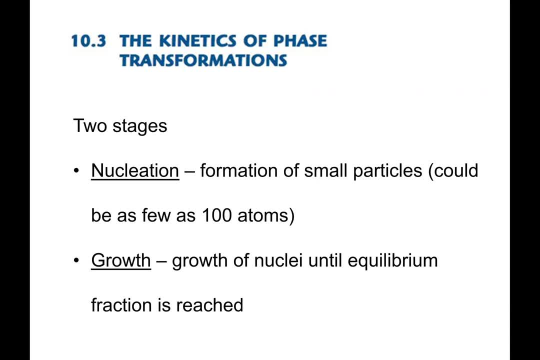 form small particles of the new phase, and this could be very small. This could be, for example, solid particles in a liquid where you are solidifying. It could be particles of perlite. so actually this would in this case be kind of a layered structure: a small amount of perlite that ferrite. 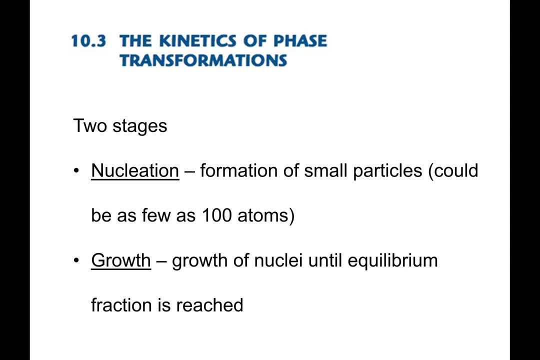 plus cementite that is forming inside of austenite. but we need to start with the nucleation of a new phase and we're going to see that there's a barrier to forming this nucleus and so that means there's going to be some rate, that is temperature dependent, that we're going. 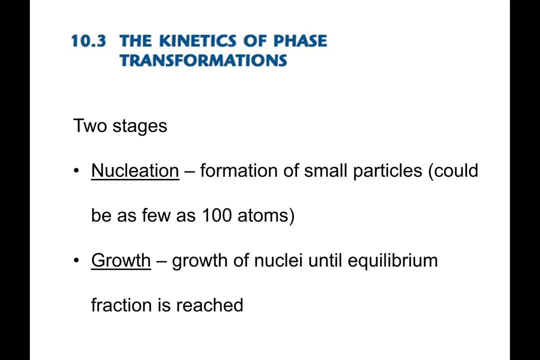 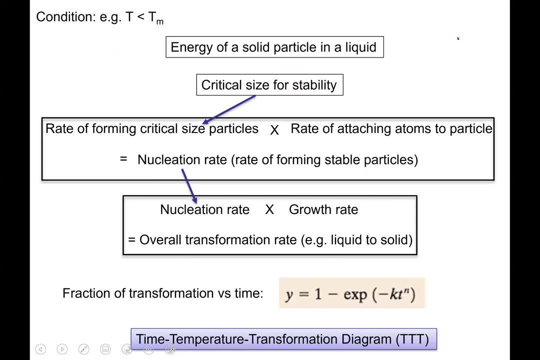 to have to look at. Once the nucleus forms. then it grows, and so we have to then look at the growth of the nuclei and to get an idea of how long the overall transformation rate will be. So there are several parts in this. This slide is a little busy, but I think it'll make more. 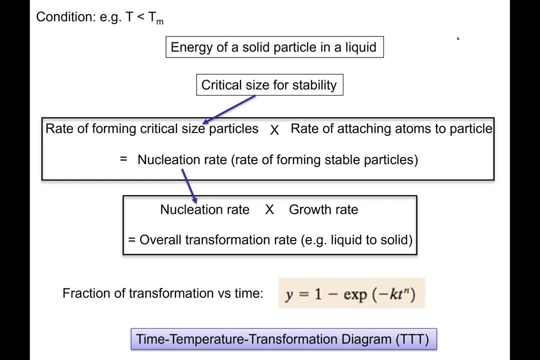 sense when we get to the end of the lecture. but it's just kind of a cheat sheet for you of the different stages that we're going to go through to get finally to the very end where we get a diagram that we can go ahead and use to predict the time. 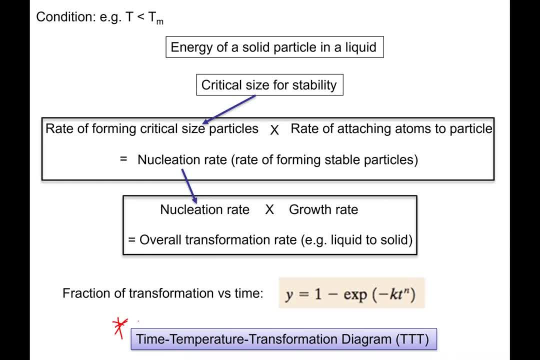 and the transformation rates. and so the idea here is: let's take a look at what we're going to do as we walk through. is we're going to go ahead and take a look at the energy for the formation of a solid particle, a nucleus? We're going to initially look at that, just for the 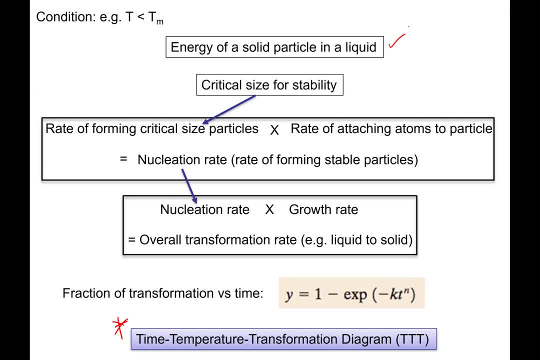 case of a liquid, but this could be any transformation in general, and when we take a look at that particle, we're going to see that there is a barrier to forming that particular particle, and so there's going to be some critical size then at which I have to get. 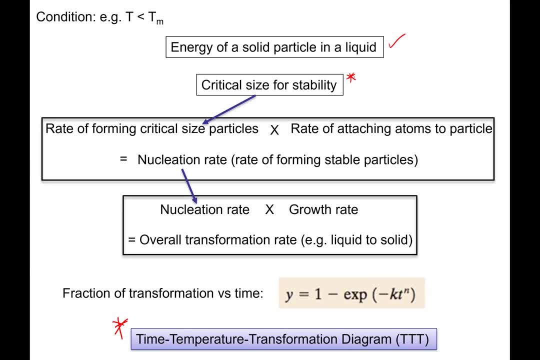 beyond in order to have stability, and then below this critical size, that particle would just simply melt again. So once I know the critical size and I have an idea of what that the energy would be for that critical size, then I can go ahead and 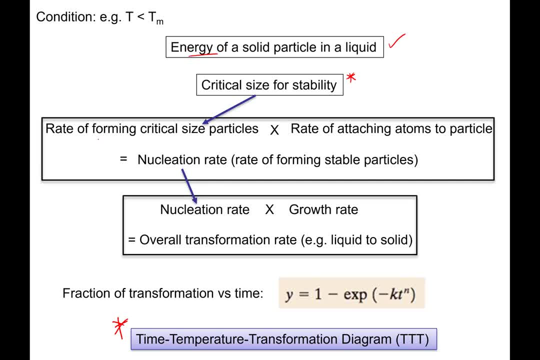 use like an Arrhenius-type equation, to find the rate at which we form those critical sized particles, And then if we can multiply that by the rate at which we attach new atoms to the particle, making it stable and growing it out, that will. 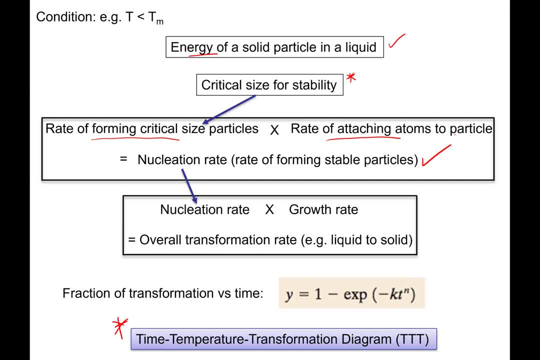 give us the nucleation rate. So what is the rate? How many nuclei per second do we form in our material? Once we know the nucleation rate, we can go ahead and multiply by the growth rate to then get an idea of the overall. 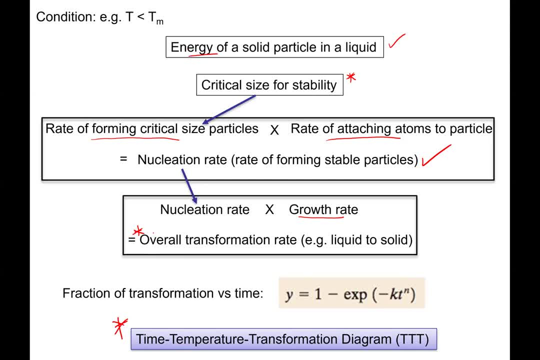 transformation rate, say, from a liquid to a solid or austenite to pearlite, And that's really what we want to get to. We want to get to this overall transformation rate, And part of going through all of this is to see the 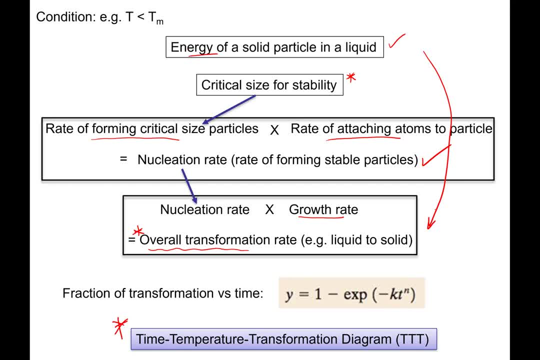 various terms that are involved, And so we're going to see how temperature affects each of these terms. So the consequence is going to be that this overall rate there's going to be an optimal transformation rate that occurs at a given temperature If we go too far above. 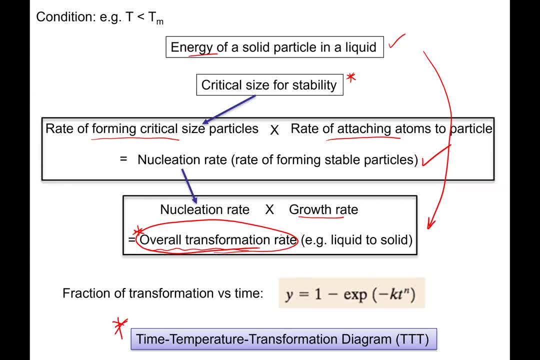 it, then our transformation rate is going to drop quite drastically, And if we go too far below it, our overall transformation rate is going to also drop quite drastically, because the nucleation rate and the growth rate are dependent on temperature in opposite directions, And so we'll see that, If we were to go. 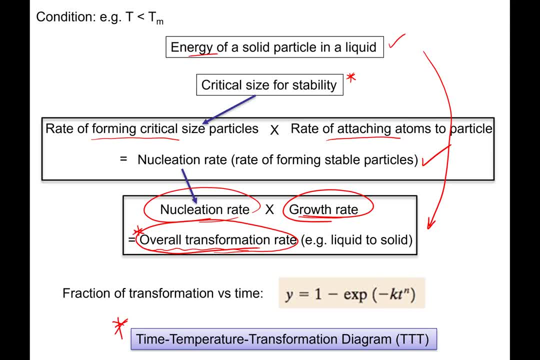 ahead and experimentally look at the transformation. so how long it takes to go from a, let's say, liquid to a solid. we were to measure that transformation at a constant temperature, we would find that it forms an S-shaped type curve. We'll look at. 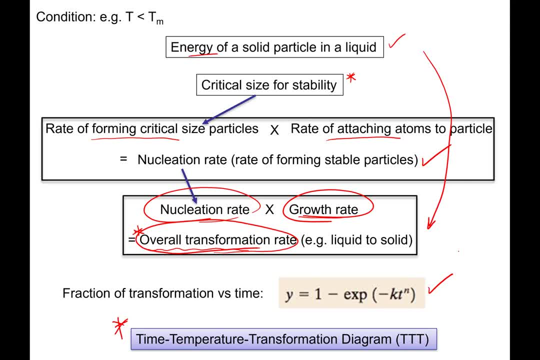 that And that's governed by this Avrami equation. So K and N here would be fits. I characterize that then ultimately, if I take a bunch of these at various temperatures, I can form finally my TTT, or time temperature transformation diagram. 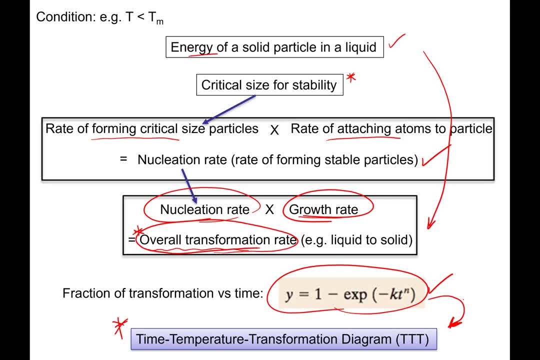 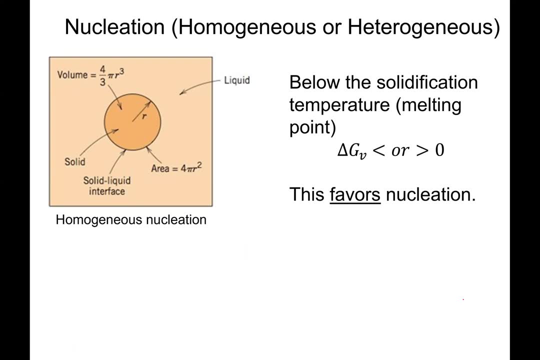 Those are going to be what we use to make predictions and estimates for transformation rates. All right, so that's kind of the process, So we're going to go ahead and move through that. So the first thing on that list was talk about the energy for forming a nucleus. 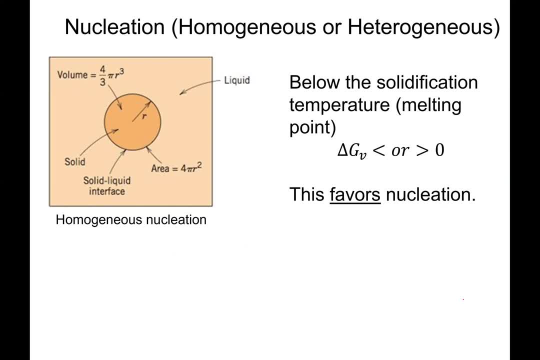 And it's trying to show you why there's a barrier to the formation of a stable particle. So the first kind of nucleation we're going to look at here is the homogeneous nucleation, And then I'll show you heterogeneous in a little bit. 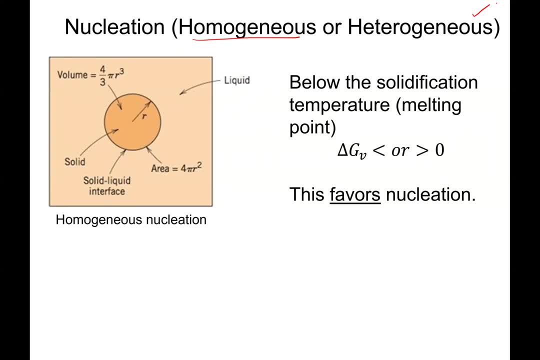 So in a homogeneous case we're going to form a spherical particle. So we've got a sphere here growing of a solid in our liquid. Maybe this is an alpha particle here in our liquid that's beginning to grow And if our temperature is below the melting point, 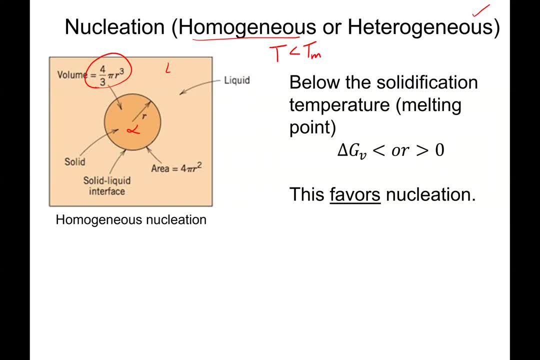 of course we need to be below the melting point or this solid particle wouldn't form. If we're below the melting point, then there is a volume free energy change that is negative, so favorable- So that's this case here- less than zero. 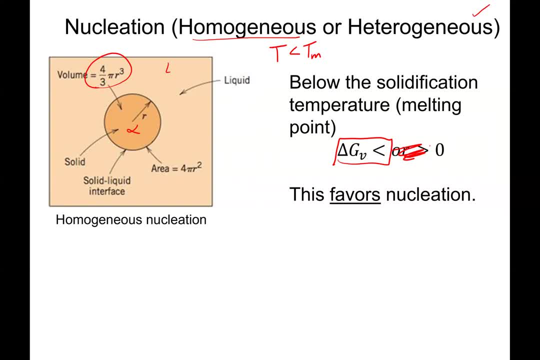 that favors the formation of the solid particle, favors the formation of a solid altogether And that's the driving force for the process. So if our free energy change per volume- so this is meant to be a, B for volume- is less than zero, 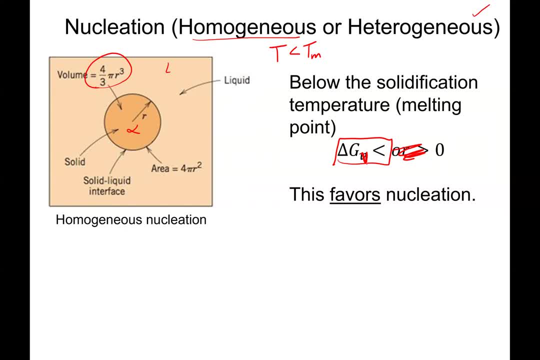 then why doesn't we just, why don't we spontaneously then just form particles everywhere and then instantly freeze? Well, the problem is is that when you form this solid particle, you've also created a defect, which is this interface, a solid, liquid interface. 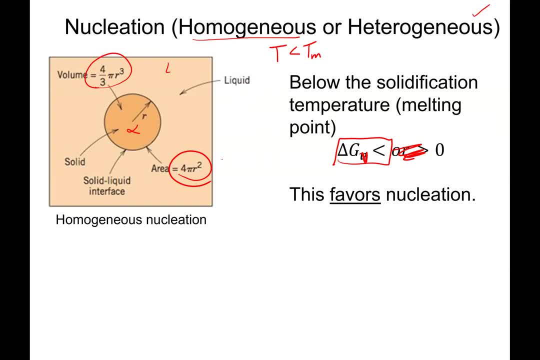 And the free energy, for that is a positive. And so we have to compare the overall free energy change for the volume transformation piece, which is a negative, and the energy gain due to forming a surface. that would be a positive term right. 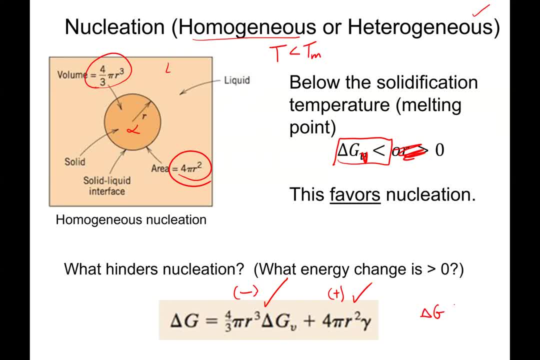 And then, overall, we need delta G in this equation here to be less than zero, to be favorable. All right, so what we're gonna actually see is that there is a critical delta G which we just simply have to overcome in order to have this transformation occur. 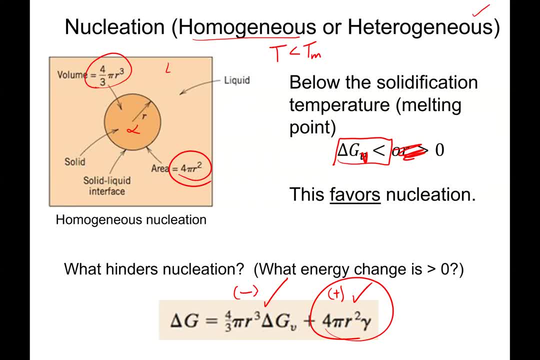 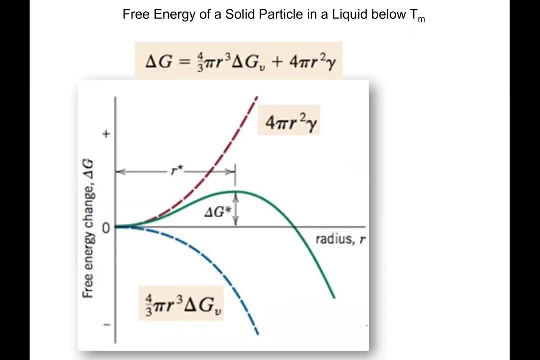 So what hinders nucleation? That is this term, the surface energy right, Four pi R squared being the surface of a sphere. So let's go ahead and look at those terms. So four pi R squared times the surface energy gamma. 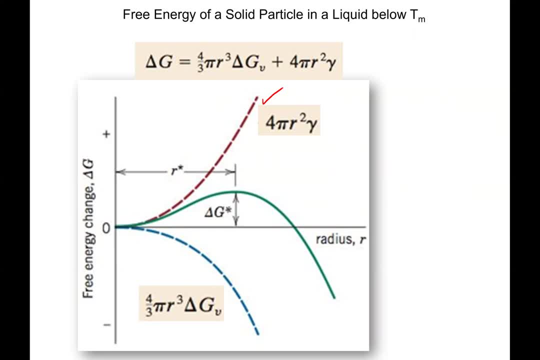 So that's a positive quantity on this free energy curve. And then we've got our volume term. four thirds pi R cubed times delta, the free energy change from a liquid to a solid, And that's a negative term. One of these terms is: like R squared one's R cubed. 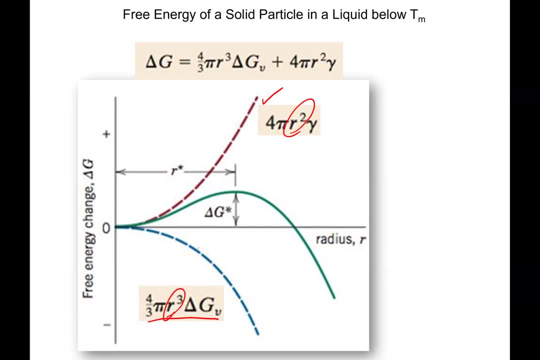 And so at smaller ends we're gonna see in this particular case that the defect energy wins, and so our overall, if we add these as positive. but as we get further away the free energy, the negative piece is gonna start winning and our curve's gonna drop. 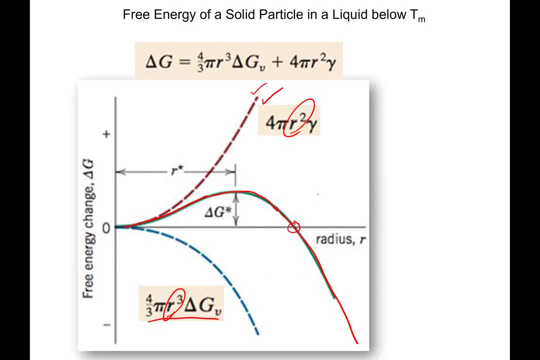 So we don't actually have to get to a free energy of zero here overall in order to have stable growth. What we actually just need to do is get past this point here up at the top, That's a star. We have to get past that point. 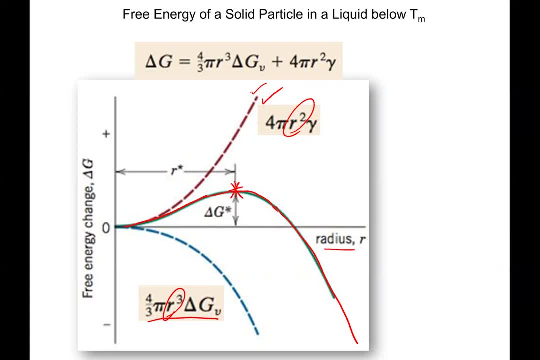 Because now, if I were to add to this solid particle, add to this radius, then I'm gonna walk this way. my overall free energy of my system is gonna start dropping, And so that's gonna be a stable particle. It's gonna wanna continue to grow. 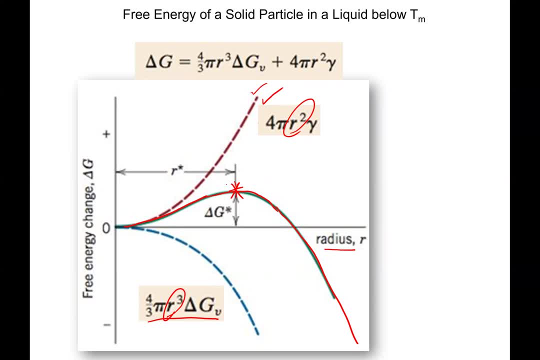 If I was a little less than that, or an atom pops off of my critical radius, then I head this way, and my free energy of my system also decreases. but this means the particle shrinks, And so we wanna figure out how many of these particles 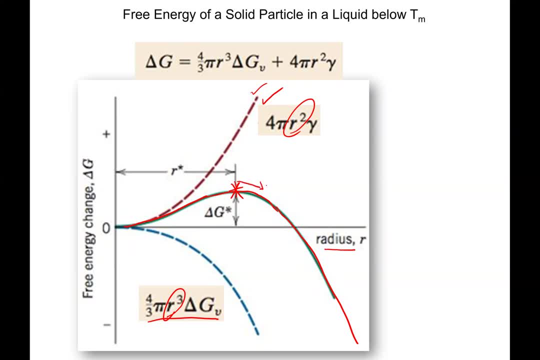 we get on this side that are stable. And then, of course, you know that in order to get these values- critical radius for the nucleus and the free energy barrier for its formation- we would get from the net equation up here and setting it equal to taking the derivative. 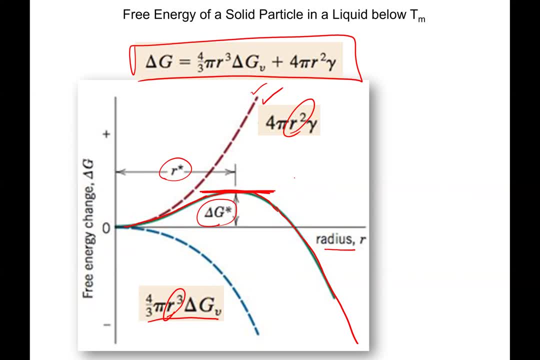 we would get from the net equation up here and setting it equal to taking the derivative and setting it equal to zero and solving for r star, plugging back in and we can get delta g star. All right, so the one thing we didn't talk about, 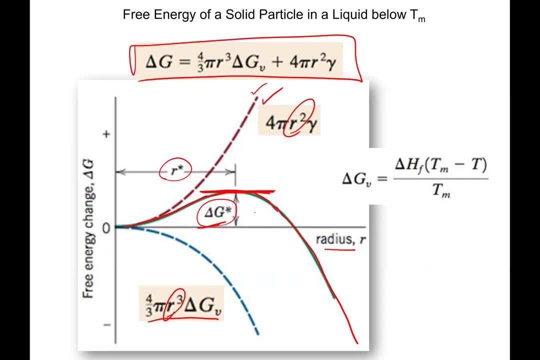 too much yet is: where does the temperature piece come in? And the temperature piece comes in due to the fact that the enthalpy term, the formation enthalpy- let me say that again, sorry- the temperature dependent nature of this comes into the fact. 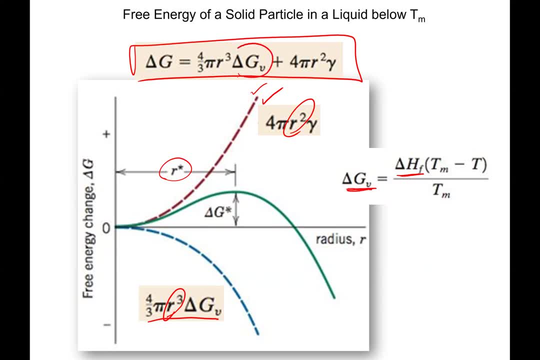 that the overall free energy is delta g. for the volume change from a liquid to a solid, which we said is a negative, is defined as the enthalpy term. This is a fixed quantity, And then it's the enthalpy times, the relative temperature to the melting point. 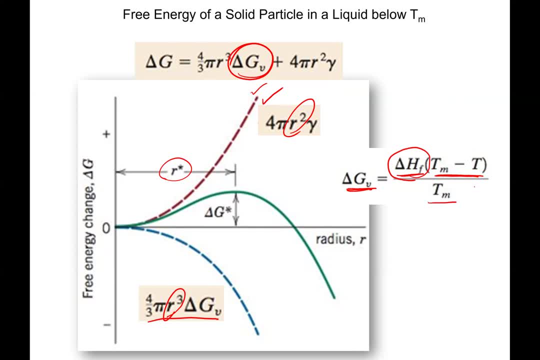 divided by the melting point. So this quantity here is a negative. So this quantity here is a negative. So this quantity here is a negative. negative when the temperature is less than the melting point. And so if I was to change the temperature, so I'm going to drop the temperatures. here's the 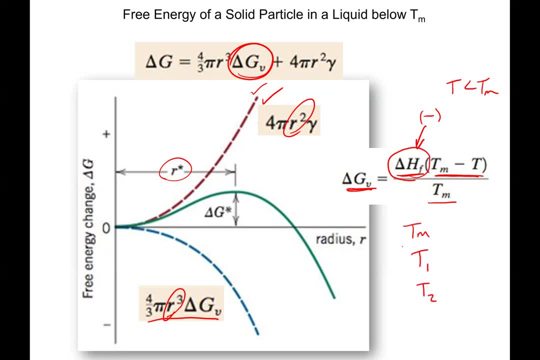 melting point. I've got a temperature T1,, temperature T2, I'm dropping the temperature down here. This curve here might represent temperature T1, and if I drop further down, say to temperature T2, my delta GV term becomes smaller. 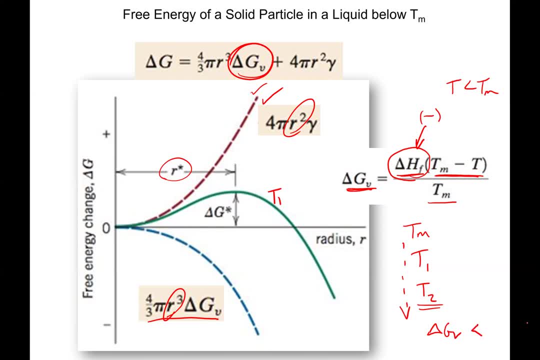 becomes more negative right, And so we've got a free energy change that's more negative and the effect is: when I take a look at the adding these curves, I'll get something like this: So this curve- free energy change curve- would shift to the left, the overall 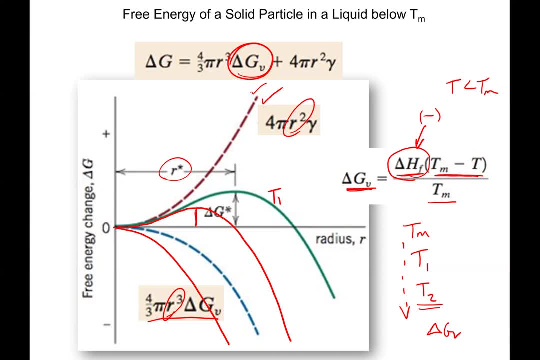 curve would shift to the left and I would end up with a smaller critical radius size and a lower barrier height, And so the lower I go in temperature, the easier it's going to become to form a nucleus. All right in heterogeneous nucleation. 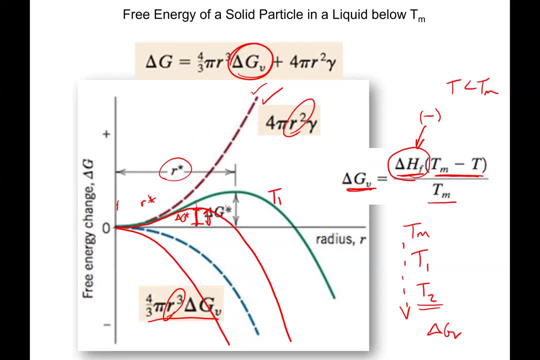 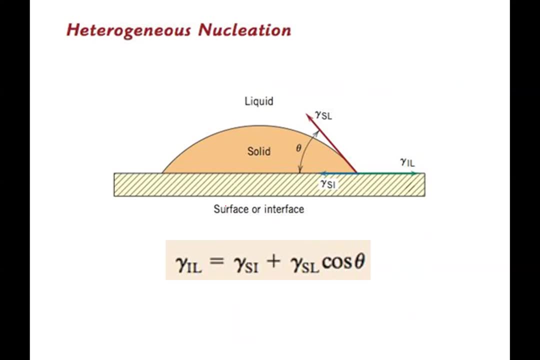 we take this negative, it Sham-GP, and we're going to form a small molecular unit here to podemos, form a liquid which we can mold on top of the liquid. And so if you're looking at the defect, like maybe the, the mold wall, and so I'm going to form now the same radius. 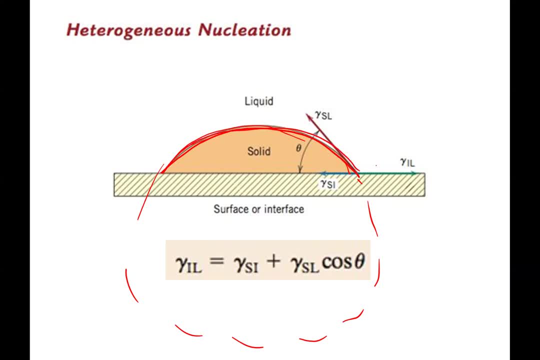 particle, but I only need this piece of it. so overall it's going to be a lower free energy but the same critical radius size. but I need fewer atoms and part of the reason why it's going to give us an overall lower energy for the formation is that is this particle forms on my, my mold. here it's going to eliminate what. 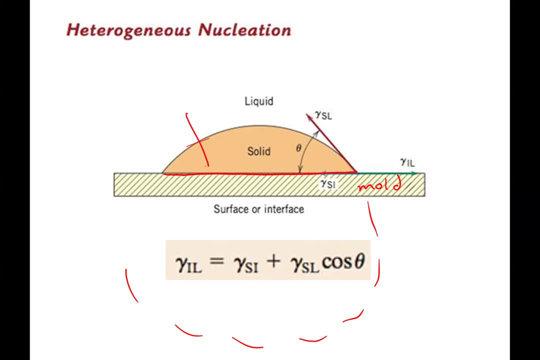 was here. now let's see draw this out. so what is here right now is the free energy related to the solid and this interface. here, what was there was an energy of the interface and the liquid, so there was already an energy associated with it. we're going to remove that. 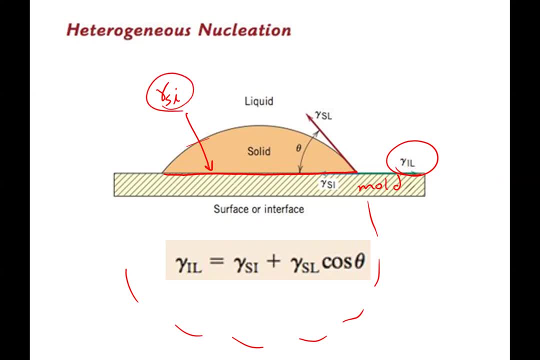 mixture from the solid point. we want to give it an equal weight and as aiesen piece and replace it with this one underneath of the particle, and so it's actually going to take a little less energy to form this particle, plus there are less atoms in it. You can read about this equation here. this helps to define. 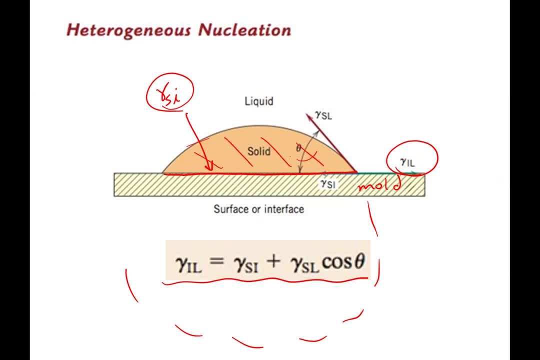 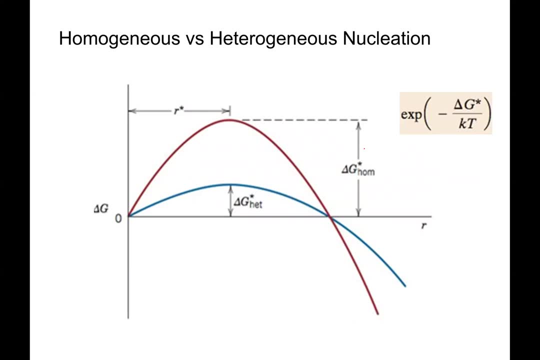 the size of this actual cap that forms by giving us a measure for this wetting angle. So here's just a schematic for the homogeneous versus heterogeneous case. you can see that for the heterogeneous case, again, the free energy drops, but the critical radius size is the same. Alright, so that means my rate of forming. 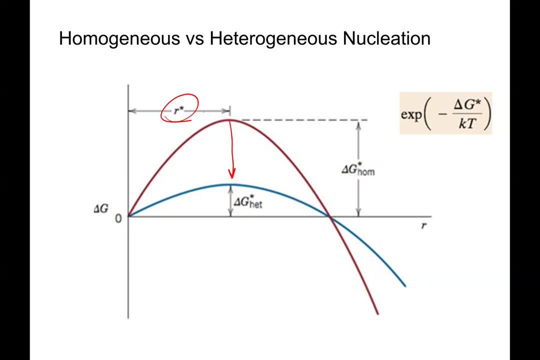 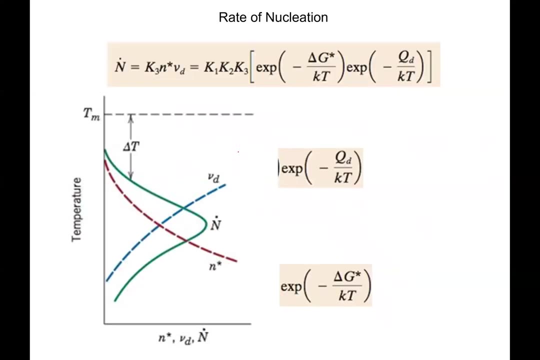 critical nuclei are going to go up significantly because, remember again, that's simply given by an Arrhenius equation. so this is the kind of the probability for overcoming this free energy barrier which we now have just dropped. but that's in the exponential. All right, so we have the rate of forming a nucleus. That was this equation I just 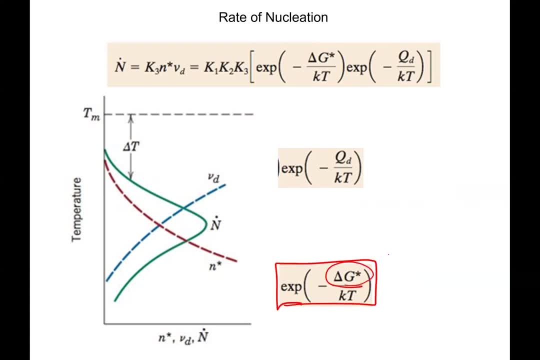 gave you. We need to overcome this barrier, whether that's homogeneous or heterogeneous, and that curve looks like this red one here. So the lower my temperature, say in the case of melting, the lower that temperature, the stronger the driving force, the smaller this delta G is because it's temperature. 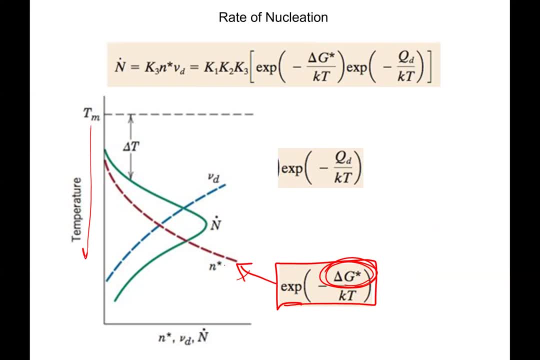 dependent, and the faster and faster my rate is going to be. The problem is that I also have to grow this particle, and so I need to attach atoms to it in order to make it a stable nucleus. This is just getting me to the critical nucleus. Well, 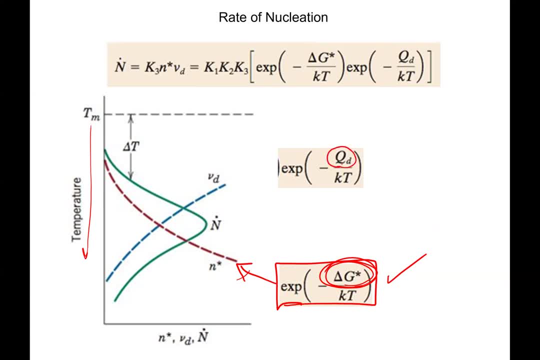 that means I've got to move atoms by diffusion. so the barrier is in the diffusion barrier and I'm going to have another rate equation that's going to describe the attachment frequency. So I just need to attach atoms to the critical and then make it stable, And so if I multiply these two together, I'm 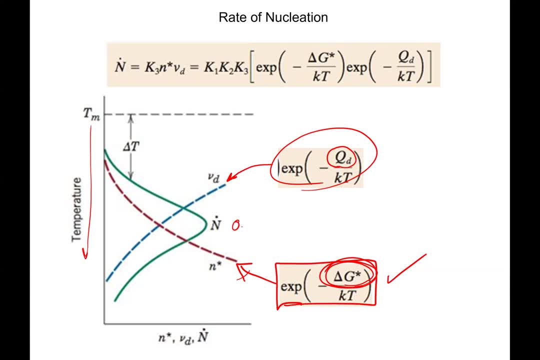 going to get then the overall nucleation rate. So this is my nucleation rate, All right, and you can see that there is a maximum value at some particular temperature here. So if I get too high in temperature I may have very rapid attachment because this curve, you know. 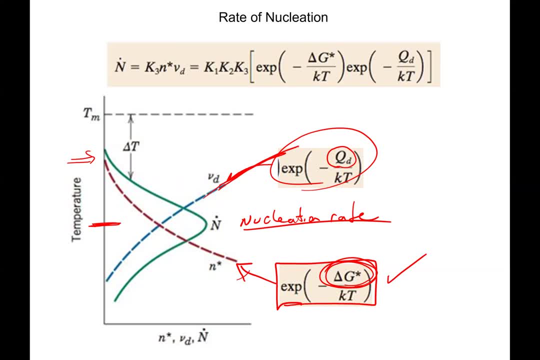 keeps coming up, very rapid diffusion to attach to a nucleus. But the problem is: from my nucleation curve you can see that I have very few and if I go too high I'll have no nuclei to actually attach to. And on the other end, if I was 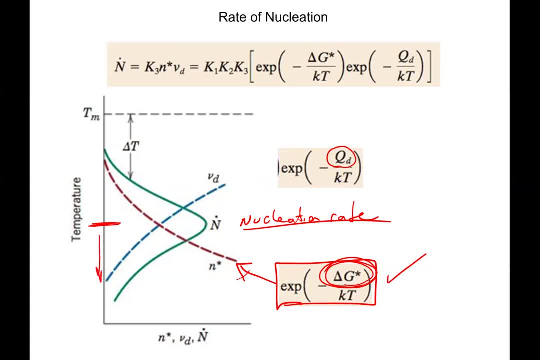 to go too far down in temperature. now I have plenty of nuclei that will want to form. Problem is is I don't have an attachment rate here to actually grow them to beyond the critical size, And so there is an optimal value then for the. 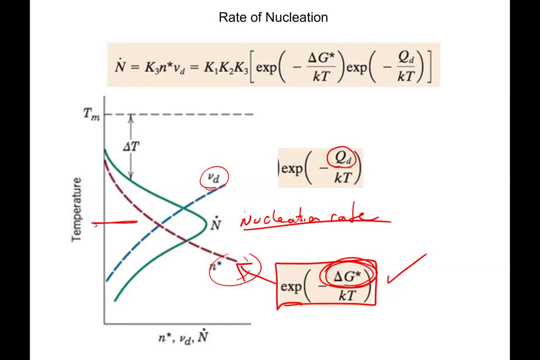 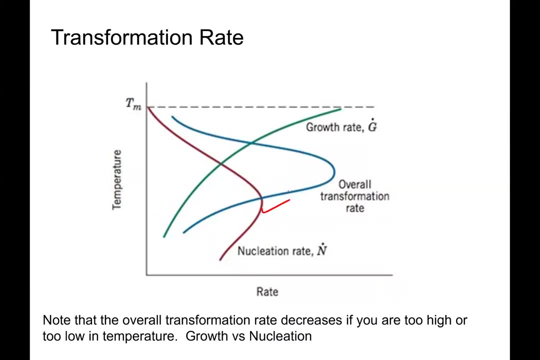 nucleation rate. All right. so that's the nucleation rate forming a critical, sorry, forming a stable nucleus. And now we need to see how quick we can grow that stable nucleus. So here's my nucleation rate that we just plotted, and then we need a growth. 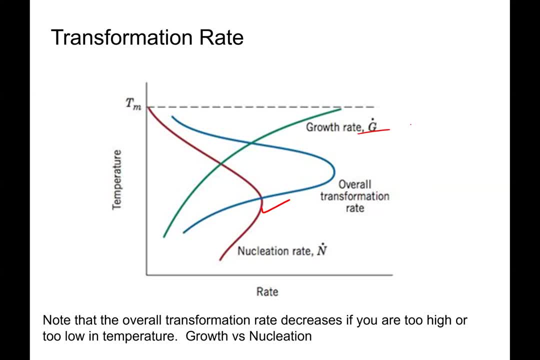 curve. So this one again is just- it's another Arrhenius that looks that has a barrier, which is simply the diffusion barrier, And so that's going to go up with temperature, because my diffusion gets faster with temperature. So the net. 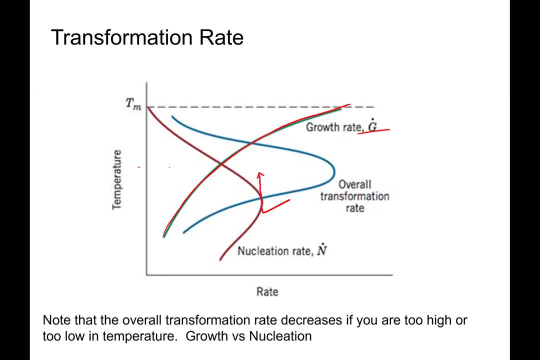 result is I'm just going to kind of shift where this optimal temperature is and I'm going to get an overall transformation rate curve. now, finally, It looks like that. So too low in temperature. my growth is too slow to grow the critical- I'm sorry- to grow the stable nucleus. too high in temperature. 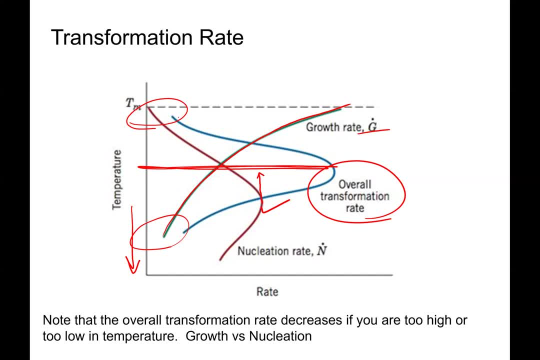 and I don't have a sufficient nucleation rate to get the process started. So, finally, in the end, this is the curve that we're interested in. this is the overall transformation rate and it shows me the nucleation rate. These are the 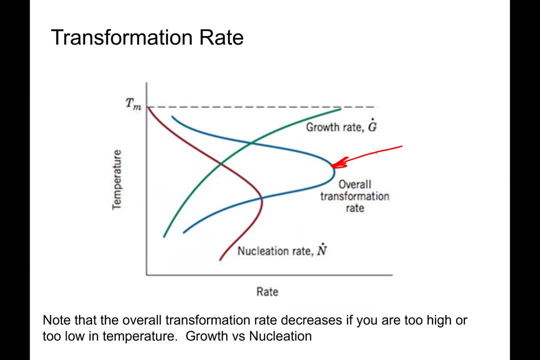 a maximum at some temperature. In the homogeneous nucleation case this difference- let's say, if we were looking at melting, you know- might be a few hundred degrees C. That's called an undercooling. So if our process of 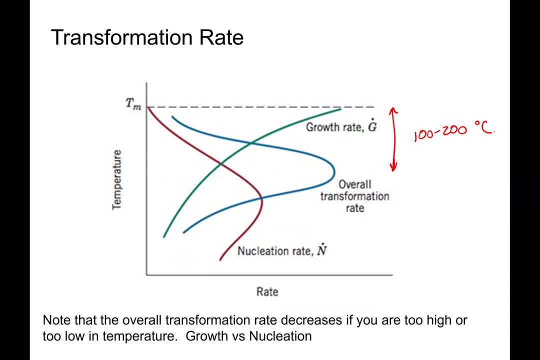 forming solids were strictly governed by homogeneous nucleation. then, to form ice, for example, you would need to be at minus 100 degrees rather than just below zero in order to get it to form, because of kinetics Once deformed thermodynamically below zero. Now we don't have to cool water down to negative. 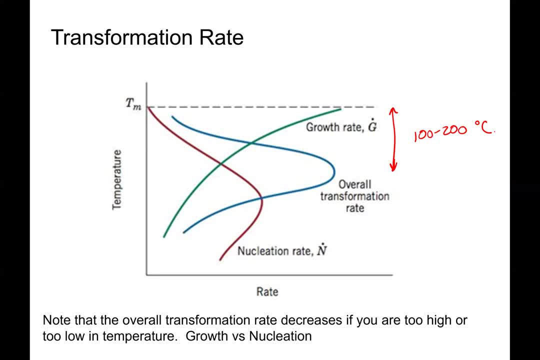 100 in order to form solid. so what that tells us is that the heterogeneous case is dominating almost all of our transformations. But we could, for example, perform this homogeneous nucleation experiment perhaps in space, where we can float the liquid and we don't have to have a container, that's. 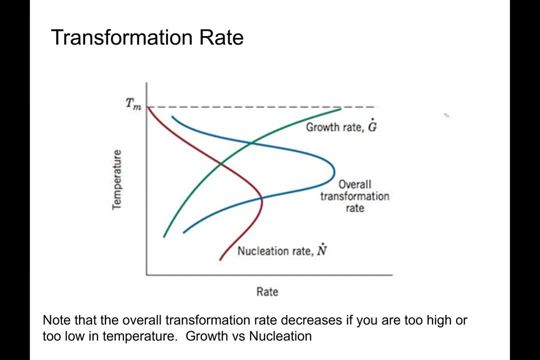 actually holding it and we can keep things pure as well. so we don't have anything in the liquid for the nucleation to start on. But the heterogeneous case is still going to have an overall maximum at some point. It's just going to be way up here, much closer to the melting point, maybe just a few. 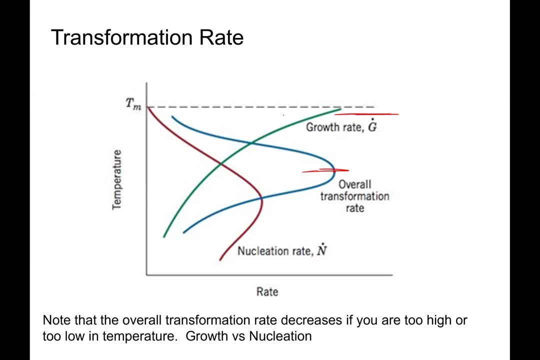 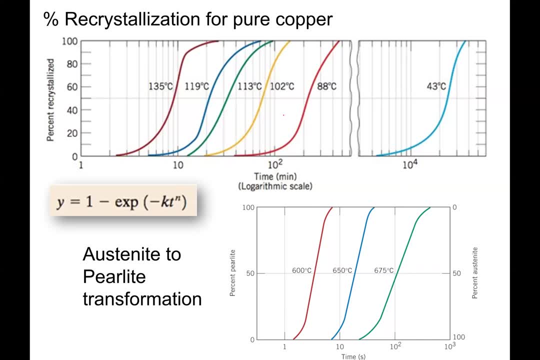 degrees below. Okay, so if we go ahead and measure now the rate of transformation at a set of given temperatures, what we're going to find is we're going to get an S-shaped type curve. So let me just kind of explain this here in a bit. This is the 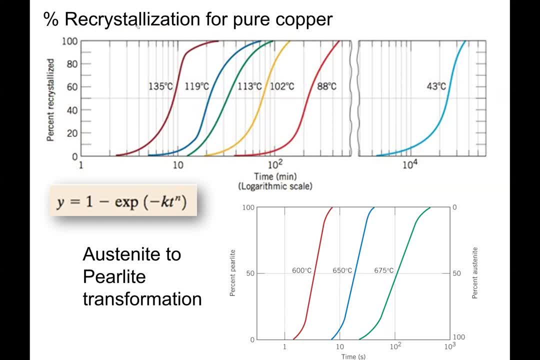 recrystallization now of pure copper. So we've put a lot of cold working in it. We've dropped the temperature down. Well, we were at the low temperature to put the cold working in it, and then we started to heat it back up. 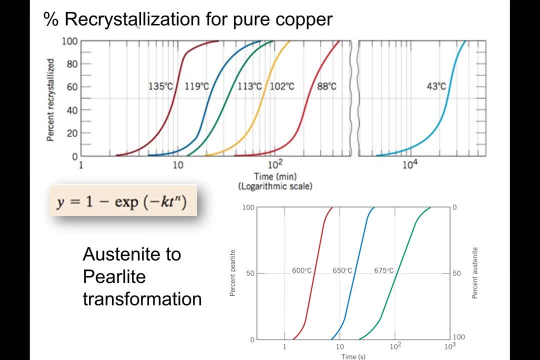 in order to get the recrystallization to start, And if I was to heat it, say to let me just pick maybe, let's say 102 degrees. So let's say I heat it up to about 100 degrees C and I watch my sample and 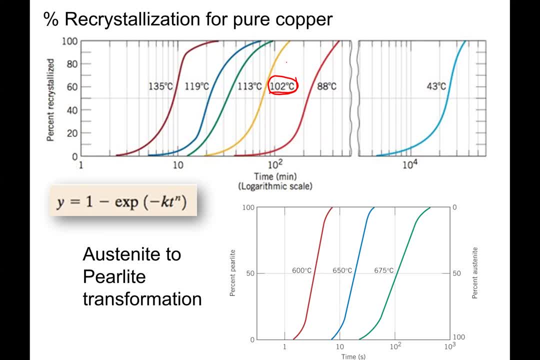 I monitor it, looking for recrystallization, what I would find is that it would take me about 20 seconds to start to see any transformation happening. So at 20 seconds I would start to see the formation of very, very tiny nuclei of new crystals. And then, if I kept waiting, 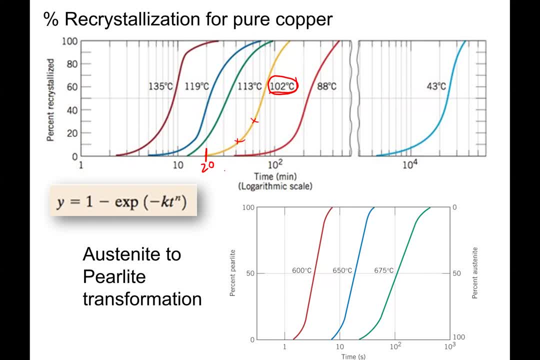 and measuring. I would find at some point that let's see 30,, 40,, 50,, 60,, 70,, 80,, 90,, 80 or so minutes that I would be 50% complete. I hope I said minutes here. It does 20. I 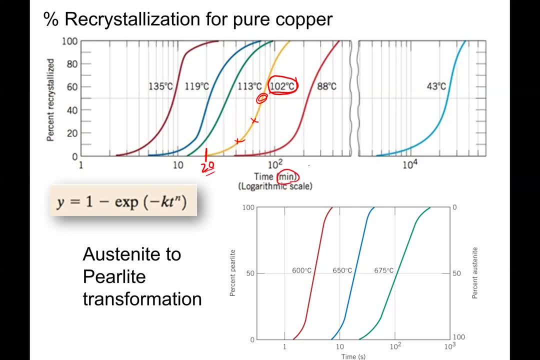 think I said seconds. This is a minute scale, So 20 minutes. it would take me to look And then if I keep watching, this curve would eventually tail back over again and I would get my time for a total 100% transformation here at about 150 seconds. 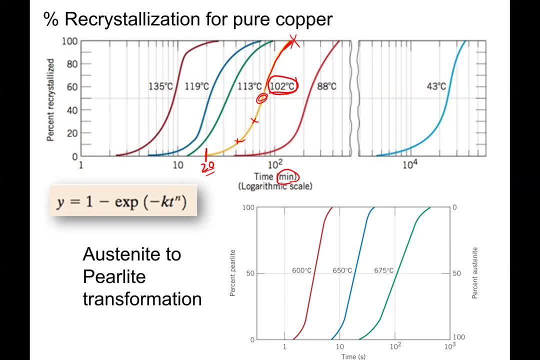 150 minutes. So somewhere around here in the middle, that's the point at which these nuclei are starting to grow out and starting to impinge on each other. They're starting to run out of- let's say, in this case, you're starting to run out of that cold worked grains. 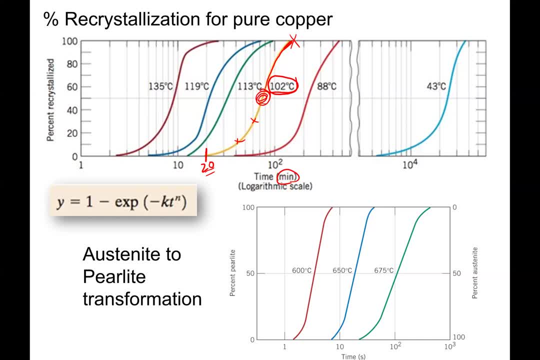 in order to transform into new grains, And so the curve has to kind of come back over again. The fastest rate is in the beginning, when they're just growing without any limitations of meeting any other grains. So that's this piece. here These S-shaped curves can be fit. 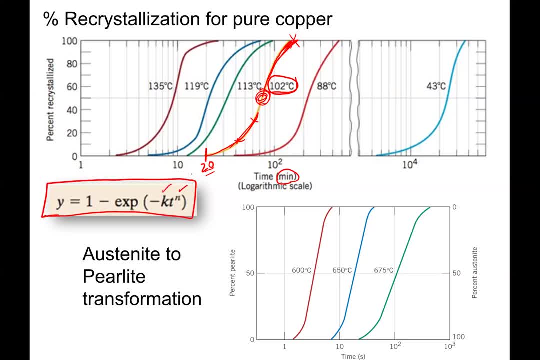 by this Avrami equation, fitting K and N, The 20 minutes here that it took for this process to start. that is our nucleation time. So that's how long it took to get enough nuclei to start actually seeing the transformation occurring. So that's your nucleation and 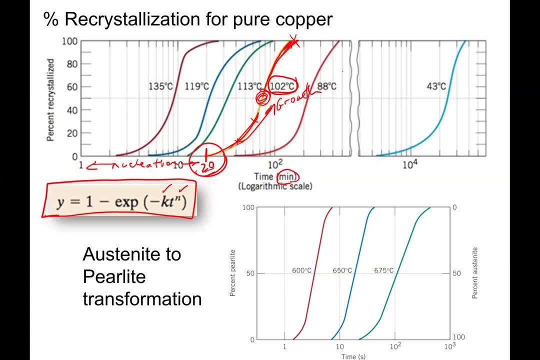 this is essentially, then, your growth That we would see in our transformation. All right, Now the other thing to notice on this one is that for the recrystallization case, when we're already at, say, room temperature and then we're heating it to get the recrystallization to occur, So I'm starting to heat, So the 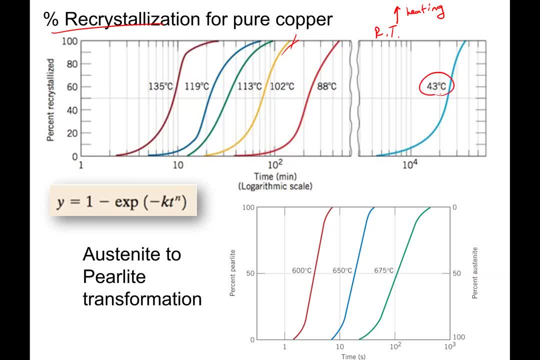 first temperature I would get to if I was to run an experiment this way, say, would be the 43 degrees C, And you can see that the time here- let's see this- is about 9,, 8,, 7,, 6, 5.. So somewhere. 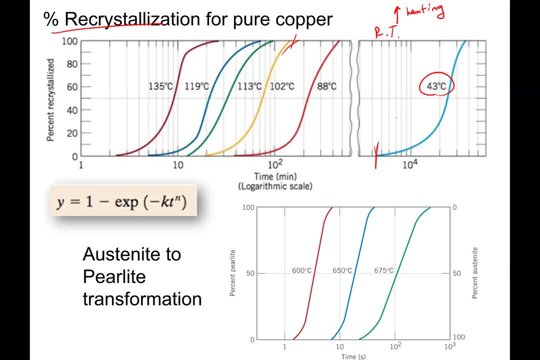 around 4,000 minutes for the nucleation to even get started, And then, as I go higher in temperature- you can see at 135 degrees C, for example- it takes a little over two minutes to start and just about 30 minutes- a half hour here- to be fully transformed. 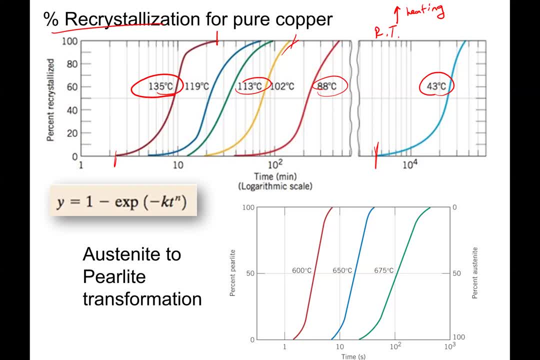 And so this transformation rate is increasing with temperature. All right, But that's not always the case. So you don't want to think that that's always the way these curves work, Because if you look at this bottom curve, you'll see that. 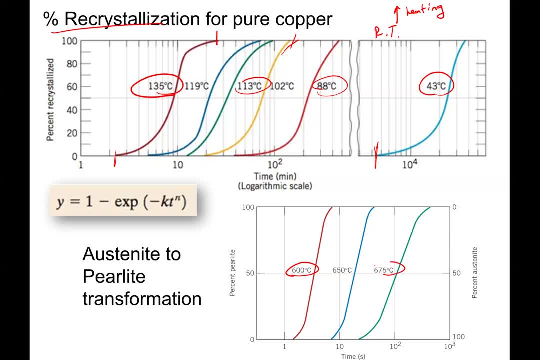 the lower temperature here is the fastest and the higher temperature is the slowest. Temperature goes like that Down here. temperature goes like this. So it depends on the direction and the type of transformation. So the bottom curve represents the transformation from austenite to pearlite, And so remember. 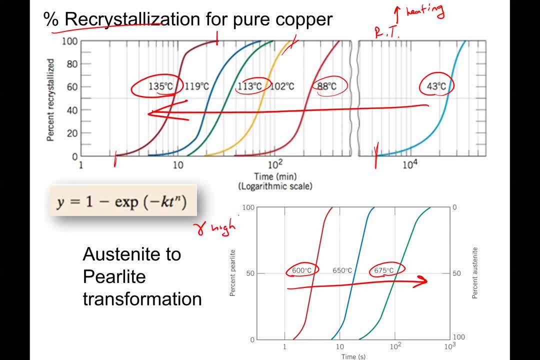 that austenite is at a high temperature And then we're dropping the temperature down into the pearlite region, right ferrite plus cementite, And so, from that perspective, the higher the temperature, the closer I am to my original gamma, And so things are going to be very slow As I drop the temperature lower and 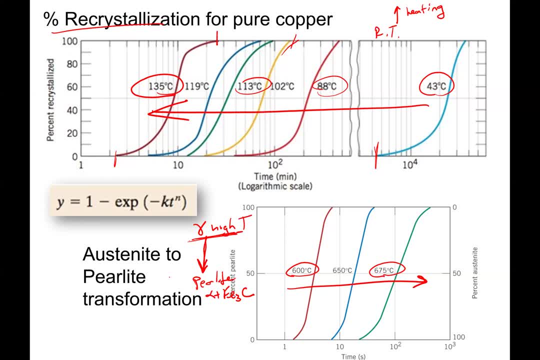 lower, I'm going to have more and more driving force And things are going to be very rapid. So here, say, at 600.. Now, eventually, if I kept going too low, then these curves would actually go the other way. They'd switch back. So, as I'm dropping the temperature down, I'm 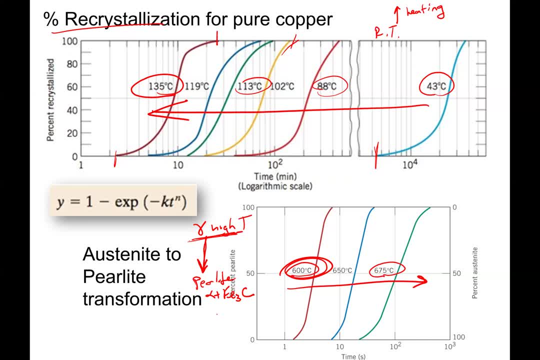 getting this faster and faster, And if I keep going down, eventually these curves would actually then start becoming slower and slower again because my diffusion would become too slow for the transformation. So I do need to try and capture that overall in a diagram so I don't have to worry about. 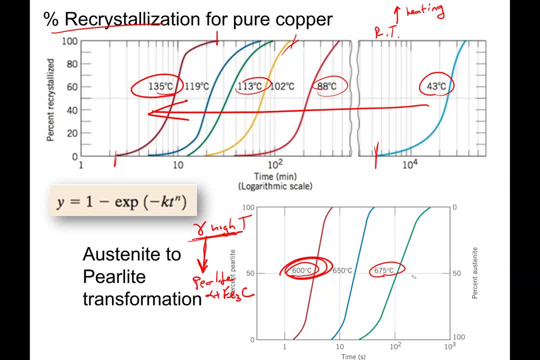 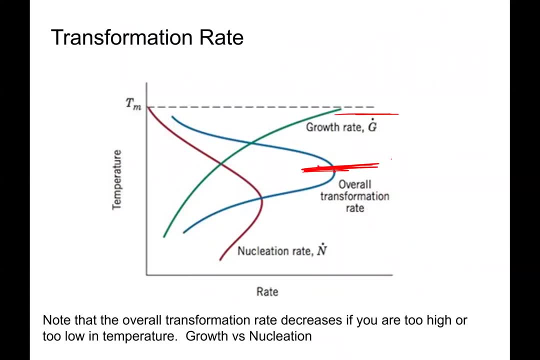 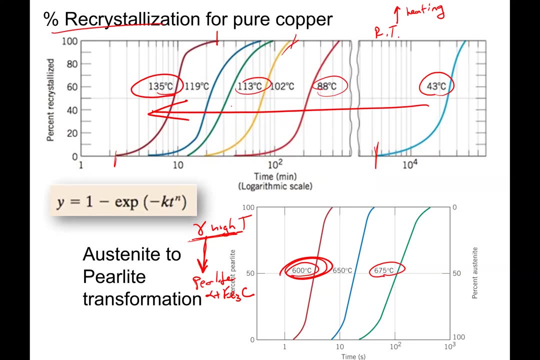 exactly where I am in terms of dropping or increasing temperatures, But this all depends upon where I am relative to this rate here. All right, All right, All right, So let's go ahead. Well, actually I'm going to do that next time, But next time what?